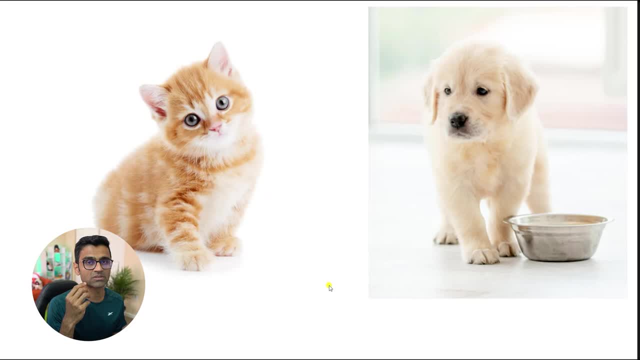 the way this works is how humans recognize these images. Or in reality. let's say you're walking on a road, You see cat coming at you or dog coming at you. How do you know it's a dog and cat and not a lion? 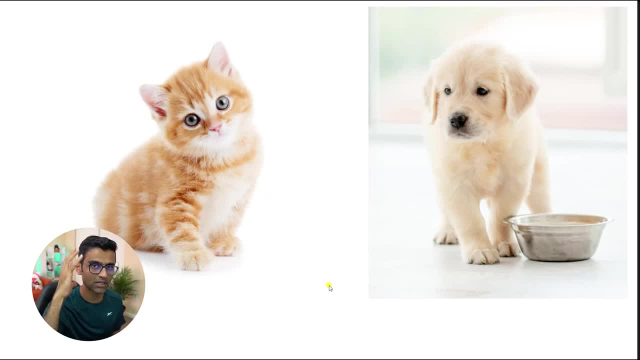 Right In your brain there is some detection happening And the way it works is: if you think about properly, is you will detect individual features such as nose. When you look at an animal and that nose, you will say, yes, it's a dog's nose or cat's nose. 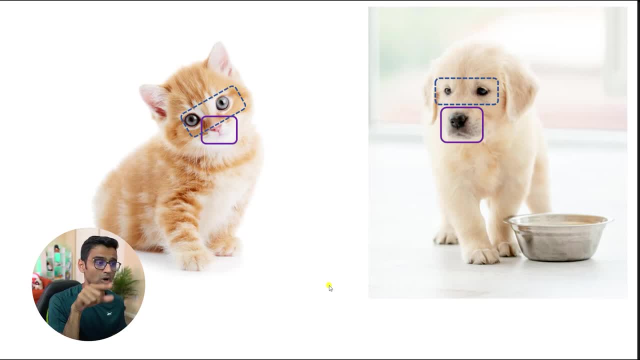 Eyes right. So you look at cat's eyes. they're round. Dog's eyes are a little different. Dog's ears are kind of falling, And cat has pointed ears, although some dogs also have pointed ears- But you get an idea that every animal has a distinct set of features. 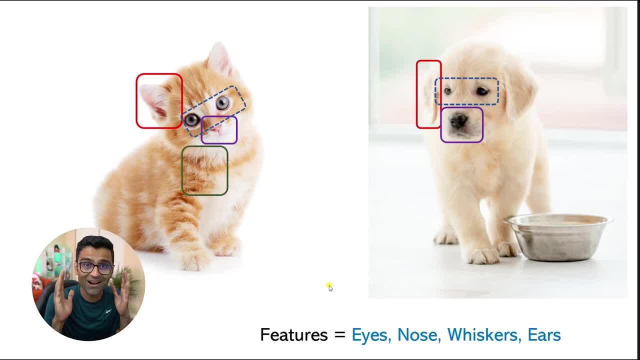 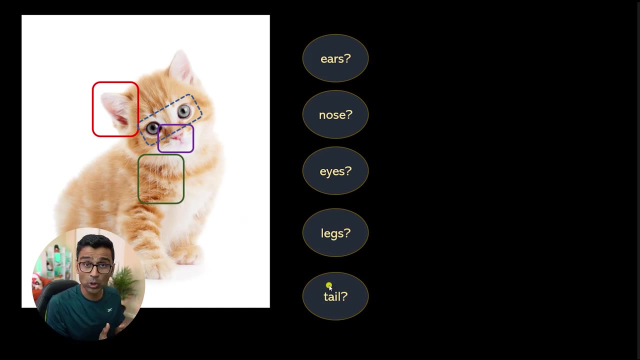 Whiskers. So eyes, nose, whiskers, ears are called features. basically Right, It's a general common sense knowledge And we use neural networks for this image classification, And I'm going to give you a very simplistic understanding of the neural network. 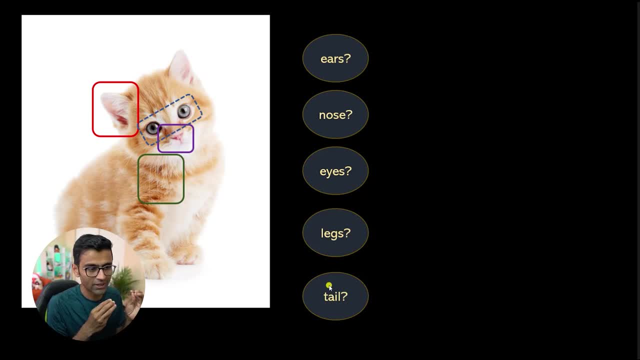 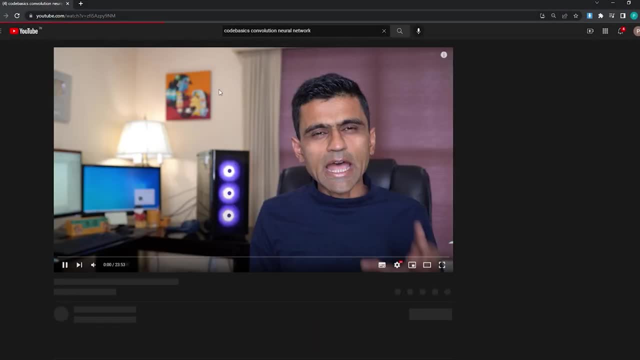 OK, this is for layman understanding. If you want to know details, in YouTube search code basics: convolutional neural network. I have explained things in detail and in a more accurate way, But this is just to give you a general idea that when you have a neural network, 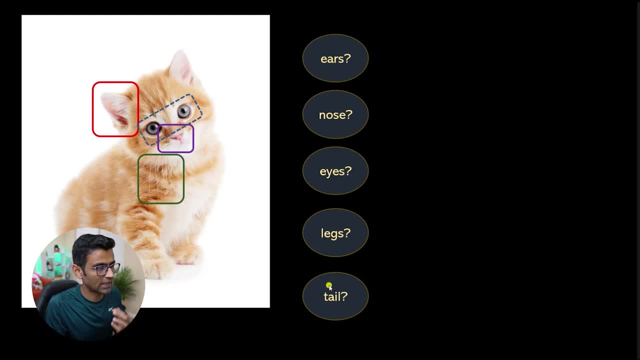 each of these neurons are like units and these units have a specific task. One unit is saying whether the ears are of cat's ears or not. The other unit is doing a task of identifying if in the image there is cat's nose or not. 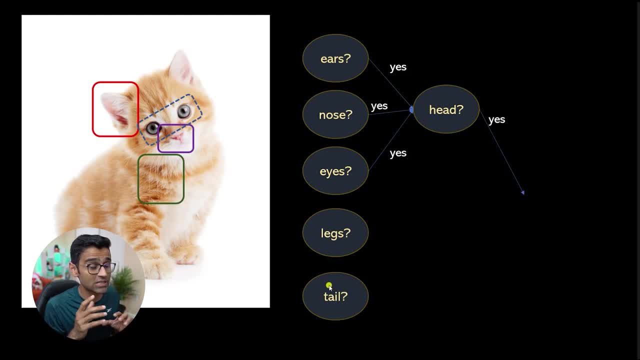 And if you get yes answer for all of this, you can say yes, In the image I have a head of a cat, And if you have a head of a cat and a body of a cat, it has to be cat. So this is how the neural network works in layman terms. 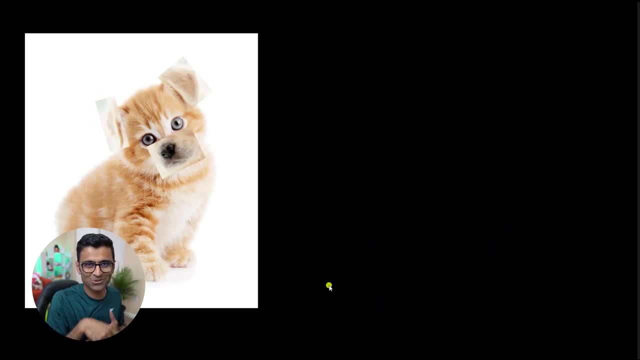 Let's say, if I show you an image like this, You know I just use Microsoft Paint and put some dog's body parts As a human. when you look at it now, you think it's cat's image, because little bit it looks like cat's. 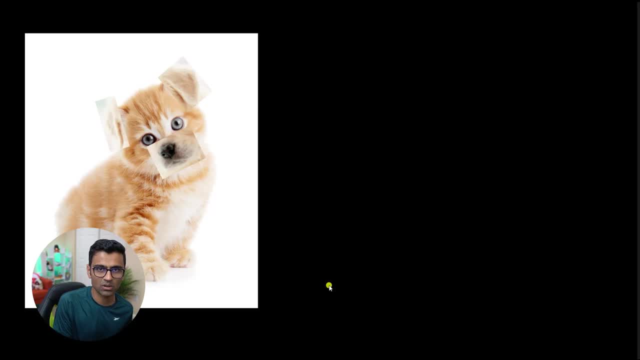 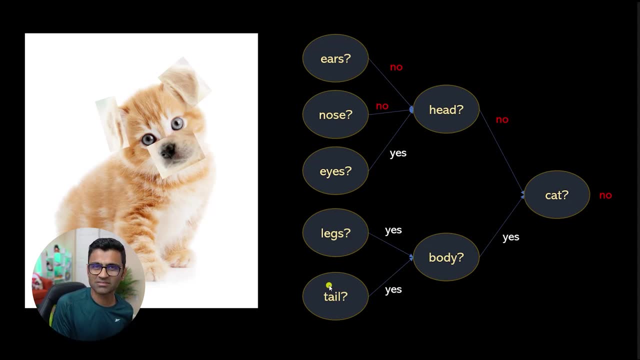 Little bit. it looks like cat's image, But you're not 100% sure Why. Because in your brain, your brain, is telling these ears and nose they don't look like cat's ears and nose. So you will say no. 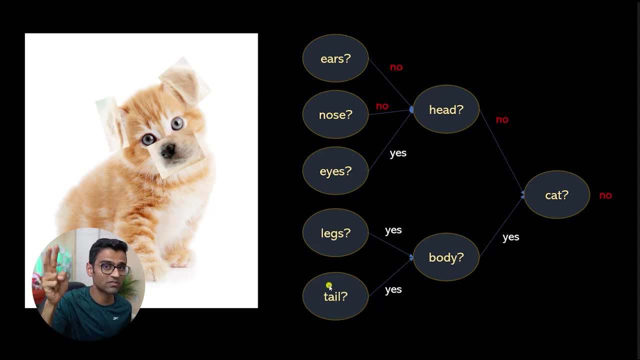 In your brain this is happening. You're saying no, no for certain features. And then if I tell you, let's say, if I remove everything and if I just show you the head of this animal in the image, and if I ask you, is it cat's head? 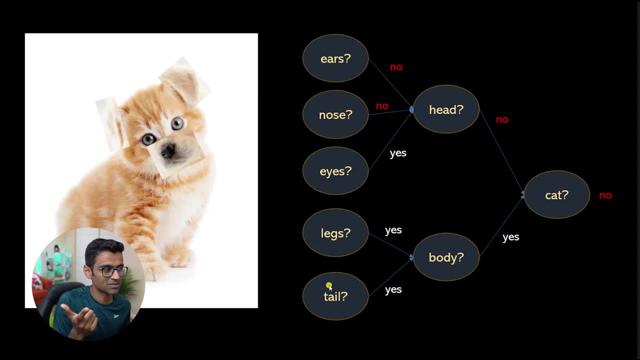 You will say no, it is not cat's head, because the ears and eyes are kind of looking different. They're not cat's ears and nose actually, Hence your overall answer might be no. Now we talked about images and the property price prediction problem, which was more like statistical machine learning. 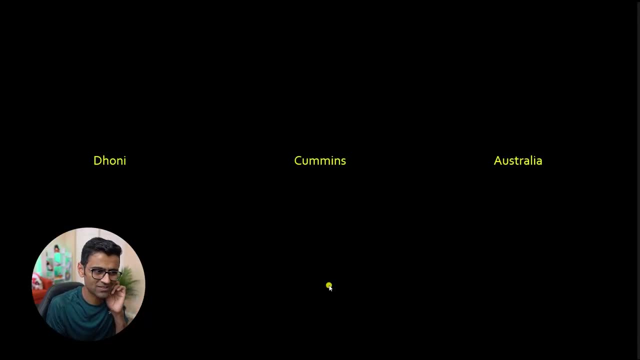 This is more like convolutional neural network. How about text? Let's say you have this text. I have given you three words: Doni Cummins, Australia. Now, if you're following cricket, you know that the first two words are actually cricket players. 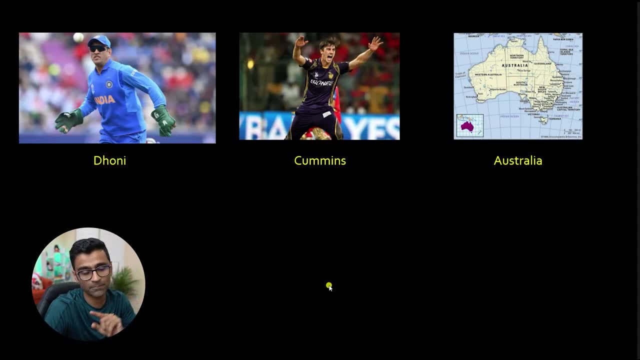 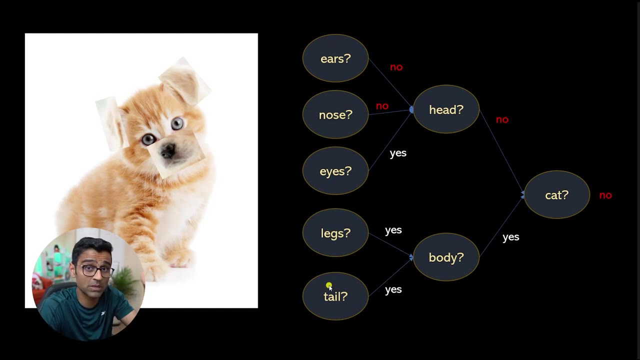 The third word is a country called Australia. How do you represent this text into features? You know how do you extract features out of it Because previously see for the image: ears, nose, eyes. they are features For property price prediction, area, location, facilities, bedrooms. 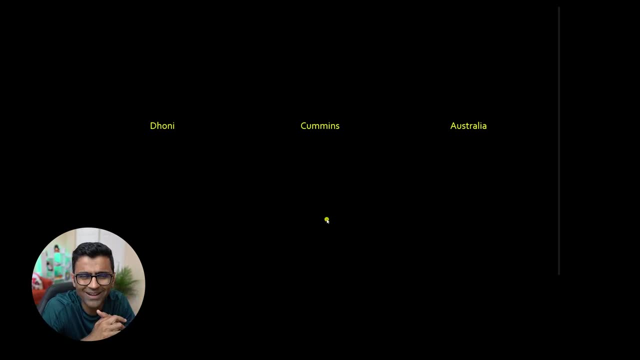 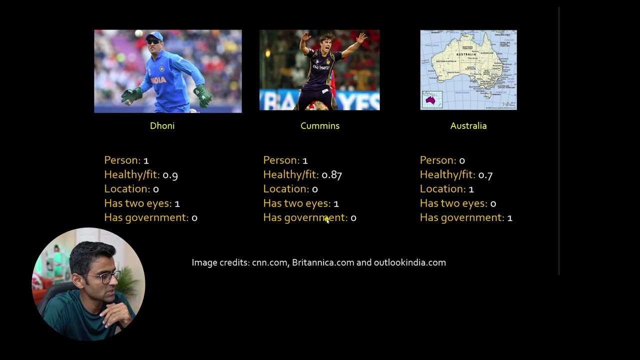 These are the features. So what are the features? for words? It seems a little bit tricky. One way could be: you can ask a couple of questions. You can say, okay, is this a person, Is he healthy or fit? Is it a location? 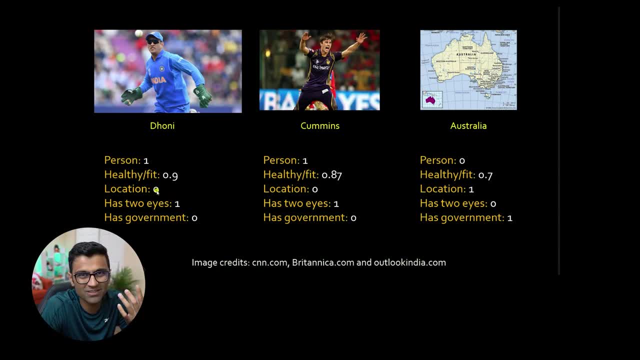 See, I have location. I have zero value means Doni is not a location, It's a person. So the value of location is zero and person is one. But Australia is a location, So value is one and person is zero. And these are like handcrafted features. 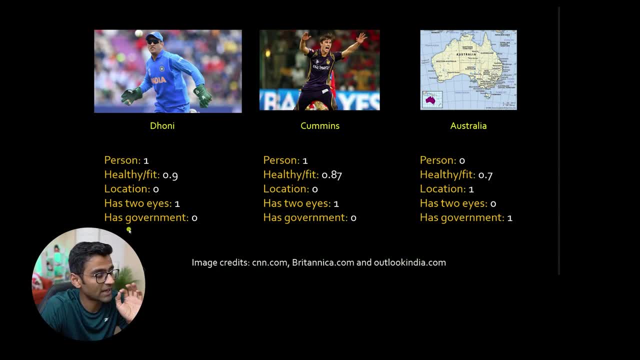 All right. So these are the features that represent these words And I can have a feature vector. So this is one of the common techniques in natural language processing where you will present a word as a vector set of numbers instead of one number. There is a reason: you don't want to assign just one single number. 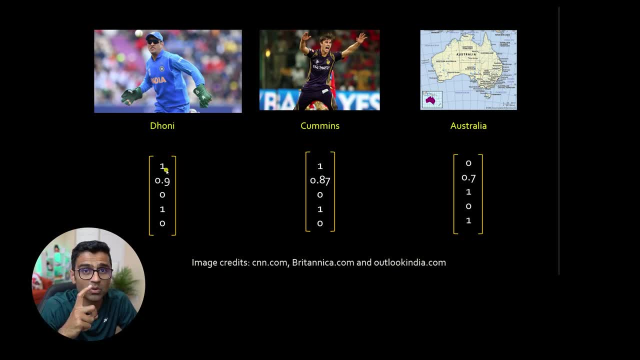 If you present it as a vector, you can do mathematical operations. Just cosine similarity. If you don't know what is cosine similarity again, go to YouTube search code: basics: cosine similarity. I have a math and statistics playlist just for machine learning. 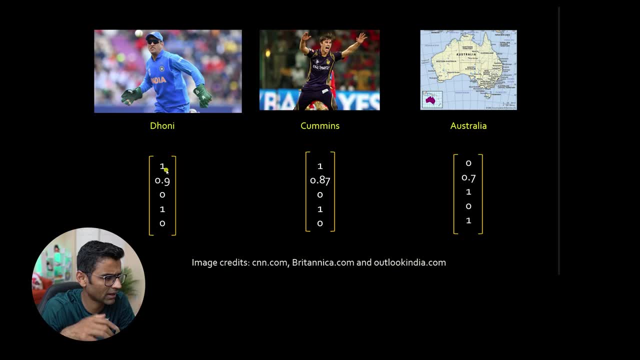 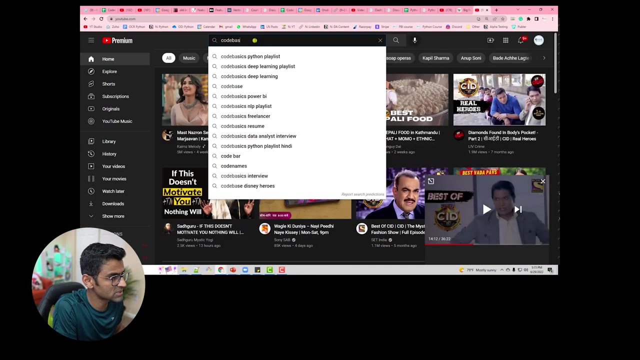 You will get your concept clear. I would highly recommend actually you watch that playlist. you know in YouTube type code basics, Or let me maybe just show you So in the YouTube. Let's say, if you type in code basics, Math statistics. 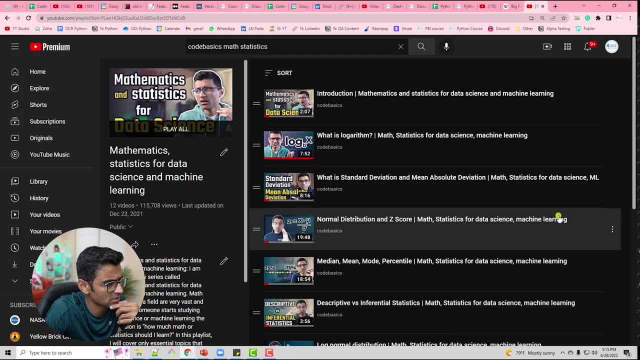 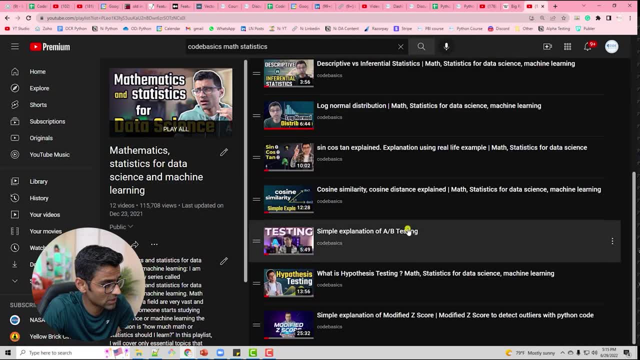 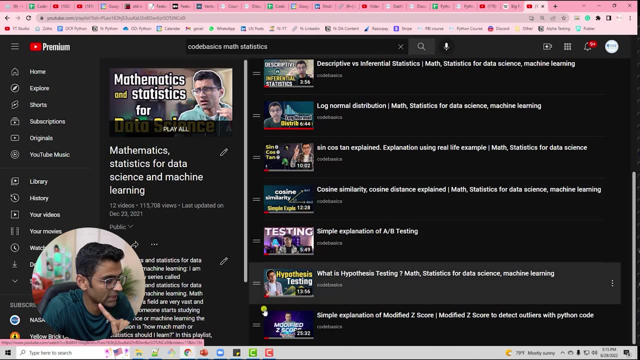 You will find this particular playlist. My wife likes to see CID, by the way, So here you will see cosine similarity And this cosine similarity, this vector mathematics, is very helpful in NLP. That is one of the reasons why we present. 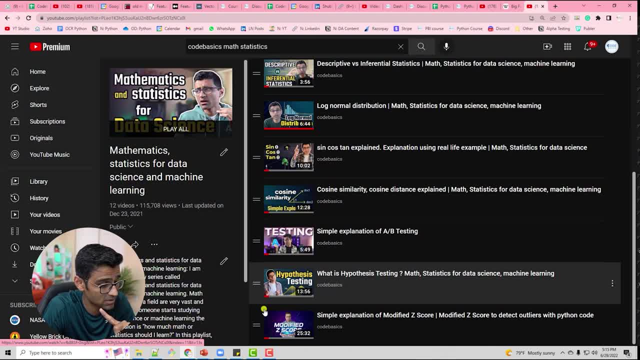 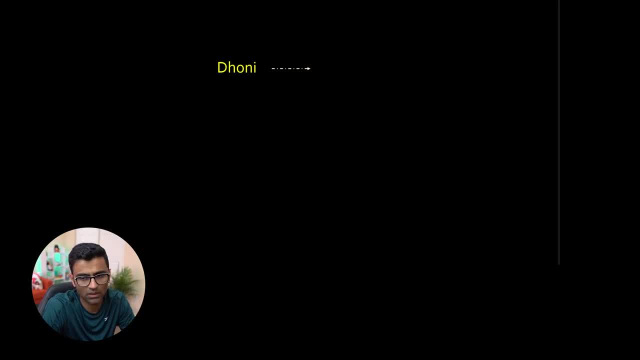 Why we present the words As vectors. All right, So essentially, what we did is we had a word, We use some technique. Now let's not go into detail. You will be like, OK, how did you come up with these questions? 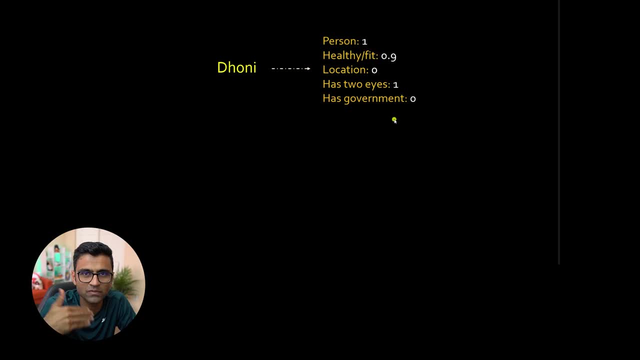 I just made it up, folks, for your understanding. OK, as we go, as we make progress in this course, you will find out. But just for your understanding, we use some criteria to come up with a vector for a word. 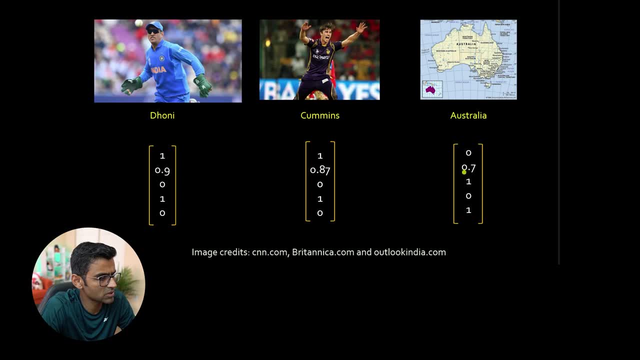 And you know there is a problem, And you know there is a benefit of doing it this way, because now, when you're comparing Dhoni versus Cummins Cummins, you will see a lot of similarity. See one one, point nine, point eight, seven: 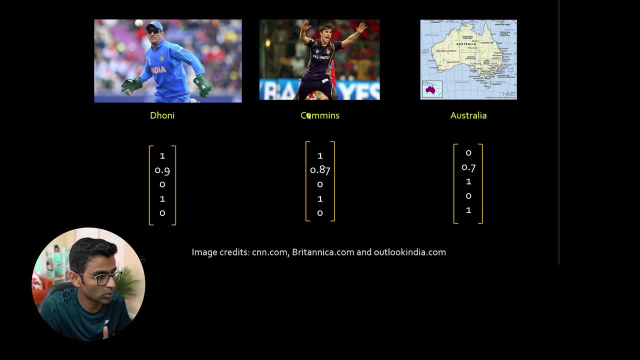 So when you do a cosine similarity between these two words, Dhoni and Cummins will be more similar than Dhoni and Australia. The cosine similarity between Dhoni and Australia will not be They want. these two vectors won't be that similar, But the vectors of Dhoni and Cummins, Cummins vectors is basically these numbers. 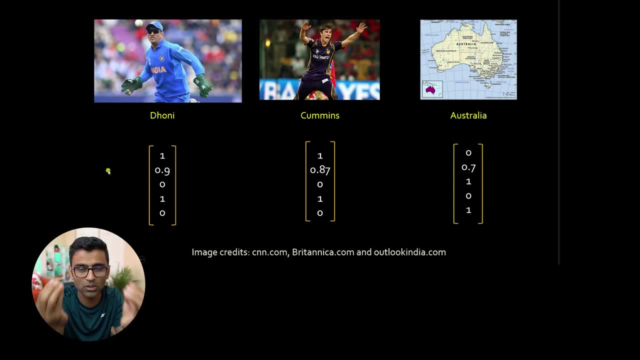 You know it's like a basic math. If you you need to know basic math, vector math, And for that I refer you to that playlist. So the cosine similarity between Dhoni and Cummins is higher. They are highly similar. 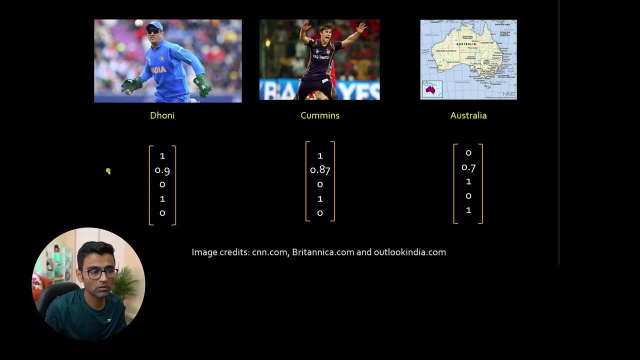 So now, when you're doing any kind of NLP, when you're working on NLP problem, having similar representation for similar words is very, very useful. Correct? You are building sentiment analysis model and you have a product review. let's say: 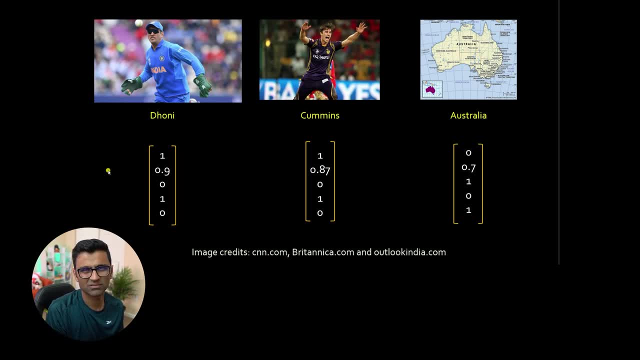 where you say The product is worse, Okay, And you have built a model based on this kind of training set. And, let's say, when you're predicting and you say, if the product is bad, now worse and bad are similar words. So if you have this kind of vectors, it will help you figure out that these are similar. 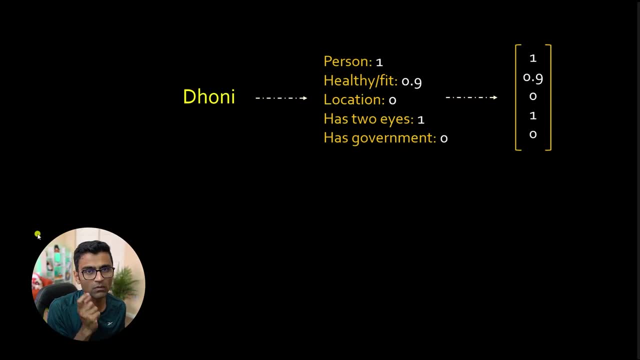 So here the idea is: you converted a word into a vector of numbers. Why do we do that? Machine learning models do not understand text. That's the fundamental thing you need to remember. Machine learning models need numbers. They can't work on text. 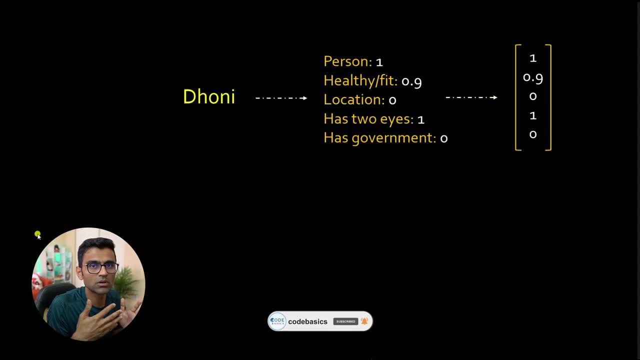 You have to convert your text into numbers, And this is one of the ways of converting text into a number, which is a vector representation. It is also called vector space model. So feature engineering is basically a process of extracting features from raw data. 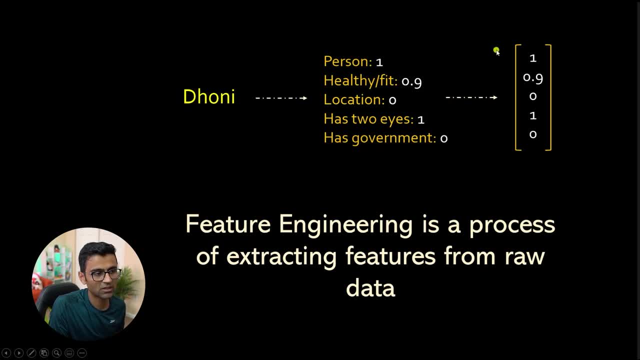 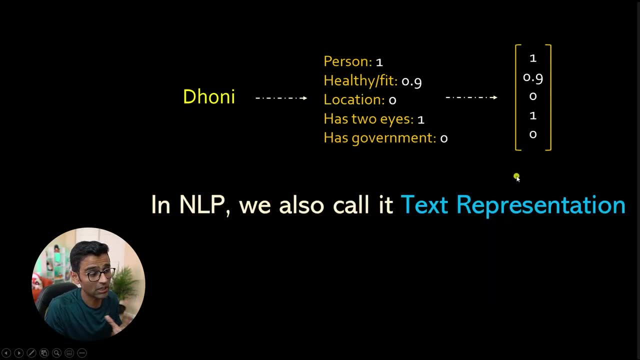 So you had raw data, which was Dhoni. You extracted all these features. You know person, healthy, fit. You constructed this vector and this process is called feature engineering. In NNP it is also called text representation. You represented this text as a vector of numbers. 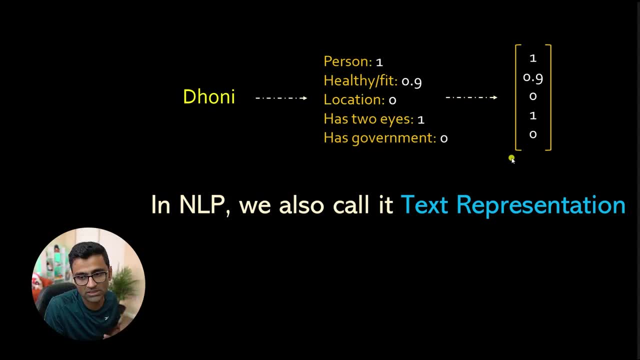 It is very simple, folks, It's not a rocket science at all. And this model, this mathematical model of coming up with a vector for a text- And when I say text, it can be word, phrase, sentence, paragraph- These are different text units. 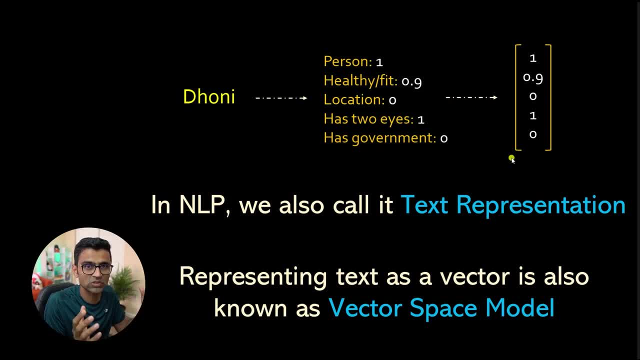 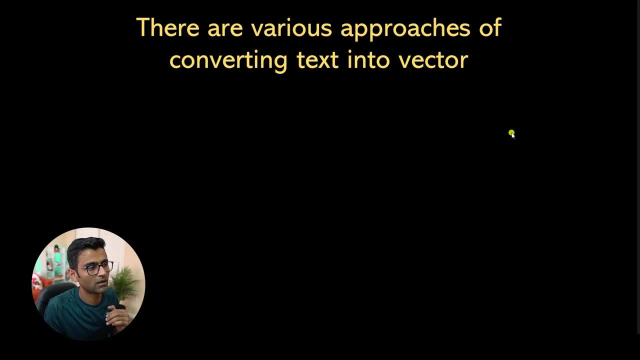 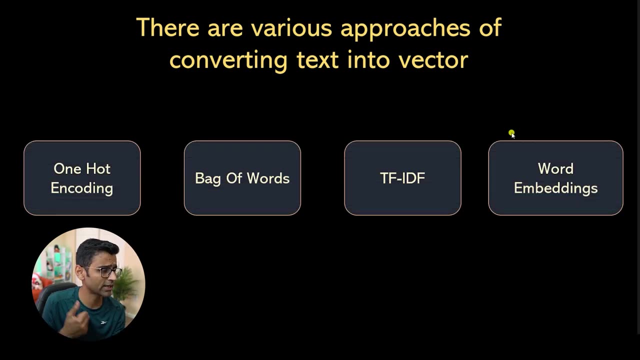 When you come up with a vector for any of these text units, it is called vector space model. Now there are various approaches of coming up with a vector for a text, Or there are various approaches of doing text representation in NLP, One hot encoding bag of words. 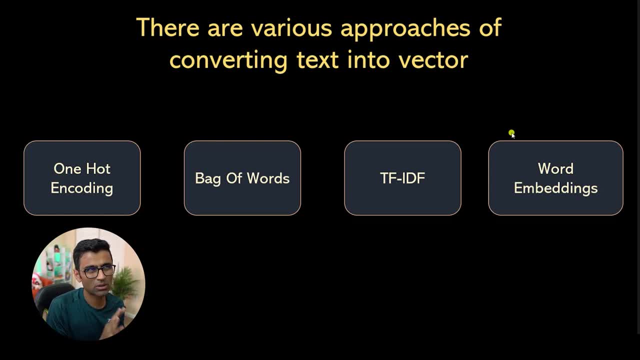 I have listed a few here. One: hot encoding is not very, very popular. I have looked into this in our machine learning playlist. If you watch code basics again YouTube, if you search code basics- machine learning, you will find my playlist. 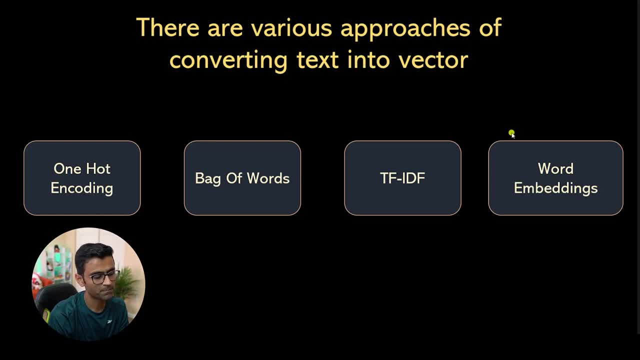 In the next video I'll tell you how many videos you need to watch. But in the next video we are going to look at most likely bag of words And we'll do coding. We'll do a classical problem of email spam detection. 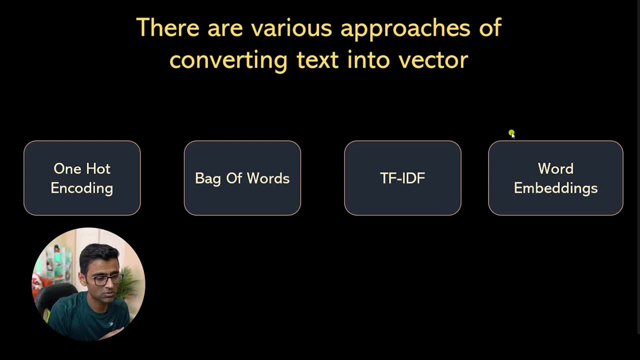 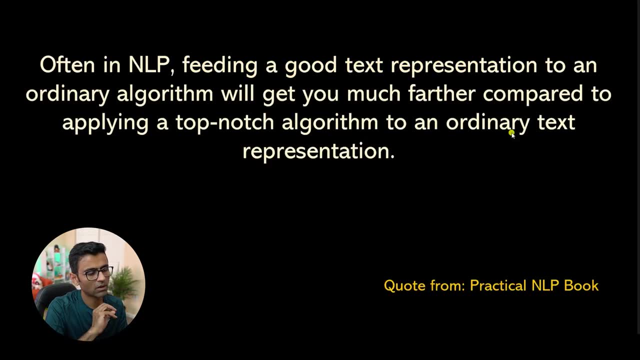 That's the agenda for the next tutorial, But in this tutorial I just wanted to give you a brief idea on what is text representation, And I want to end this session with a very important and insightful quote from this book: Practical NLP. 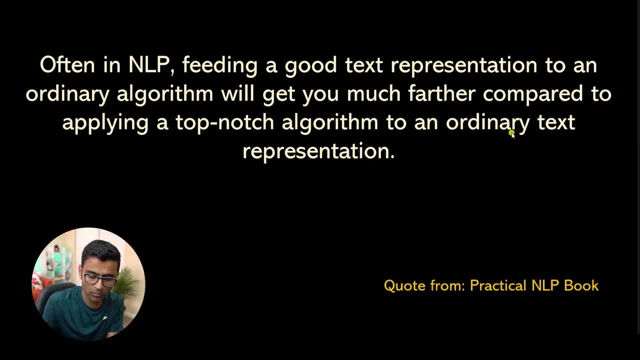 I think you should read this book. This is a very good book in NLP. The book says: often in NLP, feeding a good representation to an ordinary algorithm will get you much farther than applying top-notch algorithm to an ordinary text. So now you understand. 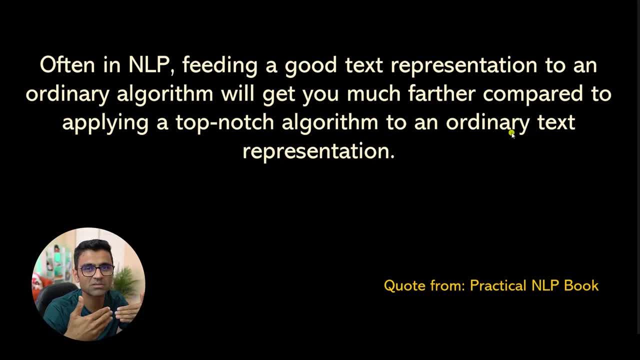 As a data scientist or NLP engineer, you should not be obsessed about what exact machine learning model you are using. You should put more focus on the text representation, See if you can extract the features in a better way from the text and if you can represent text in a good way using vector space model. 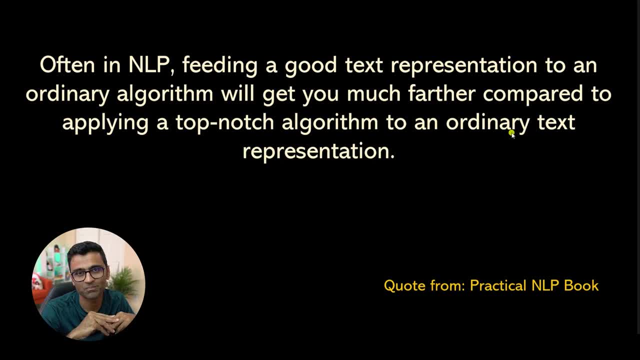 it is going to take you very, very far. I hope you liked this session, If you did give it a thumbs up. If you have any questions, post in the comments box below. In the next video we'll do coding, we'll do emails, spam detection and we'll use bag of words.